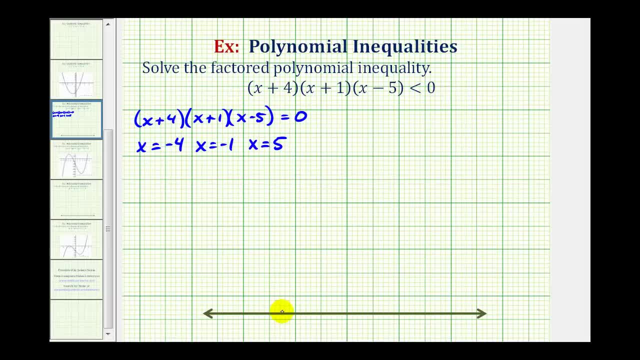 So when we plot these points on the number line, we're going to make open points to show that these are not part of the solution. If this was less than or equal to, then these values would satisfy the inequality and we'd make closed points. 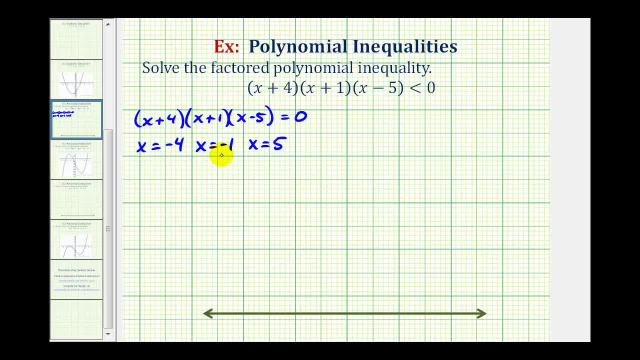 But because it's less than we're going to make open points on negative four, negative one and positive five. Notice, by plotting these three points, we now have four intervals to test. We have the interval on the left, this interval here, this interval here. 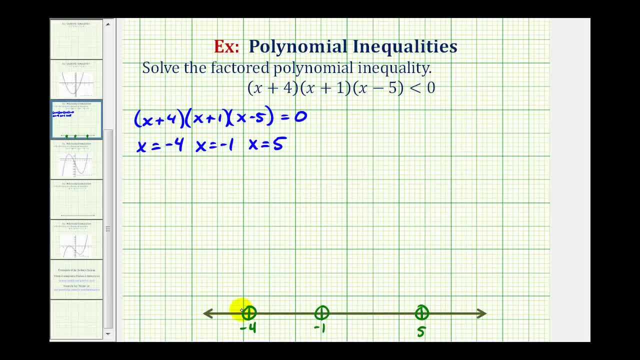 and the interval on the right. So now what we're going to do is pick test values in each interval and see if it satisfies the inequality. If the test value satisfies the inequality, the interval is part of the solution. If it doesn't, the interval is not part of the solution. 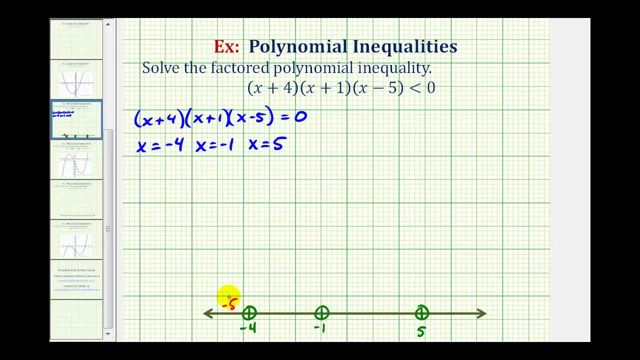 So let's test: x equals negative five to the left. And here let's go ahead and test negative two. here we'll test zero, and here we'll test six. When x equals negative five, here we'd have negative five plus four, that's negative one. 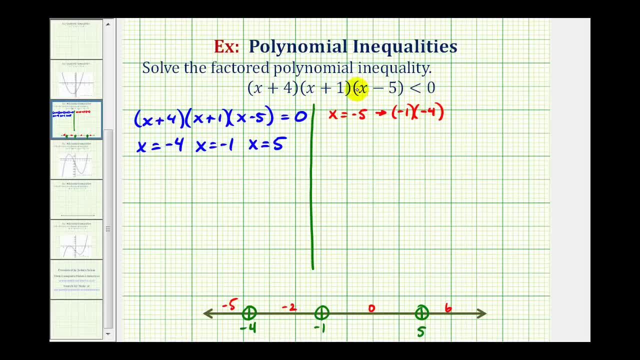 Negative five plus one is negative four And negative five minus five is equal to negative ten. We want to know if this is less than zero. This will be negative forty. Notice how we have an odd number of negatives And negative forty is less than zero. 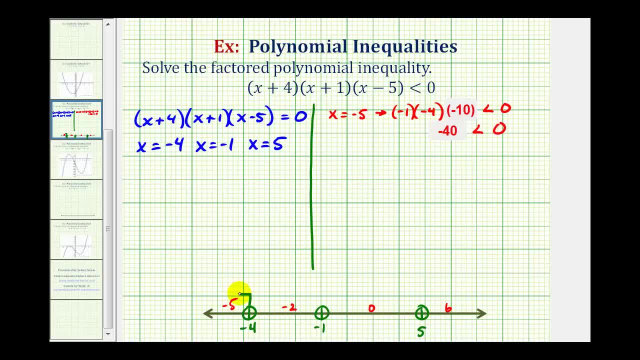 which means this interval here is part of the solution. Let's go ahead and graph it. Next we'll test: x equals negative two, So we would have negative two plus four, that's two Negative. two plus one is negative one Negative two minus five is negative seven. 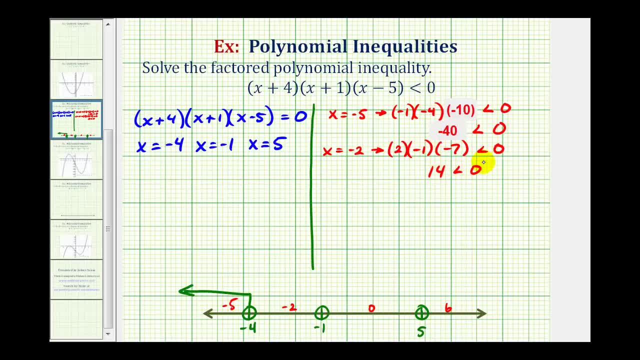 Well, here we have: positive fourteen is less than zero. that's false, Which means the interval from negative four to negative one is false. Let's go ahead and just write that in there. it's false. Now we'll test. x equals zero. 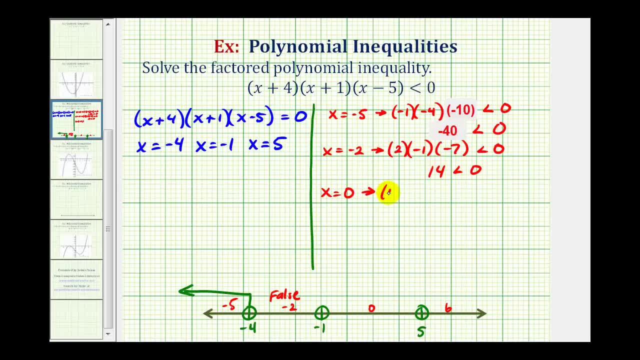 Well, when x is zero, we would have positive, four times positive, one times negative, five less than zero. This is negative. twenty is less than zero, which is true, This is true. this interval here is part of the solution, So we'll go ahead and graph that. 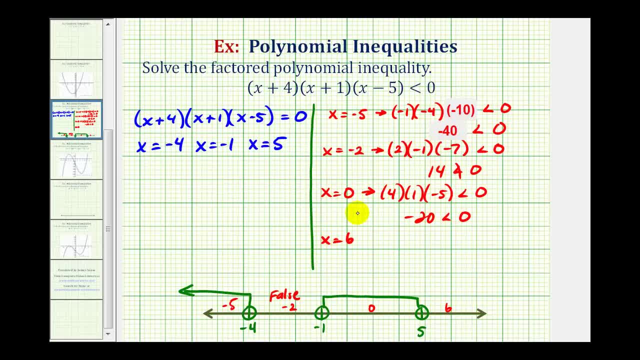 And now the last test value was: x equals six, So we'd have six plus four, that's ten Times six plus one is seven Times six minus five is one, So it looks like we have seventy is less than zero. that's false. 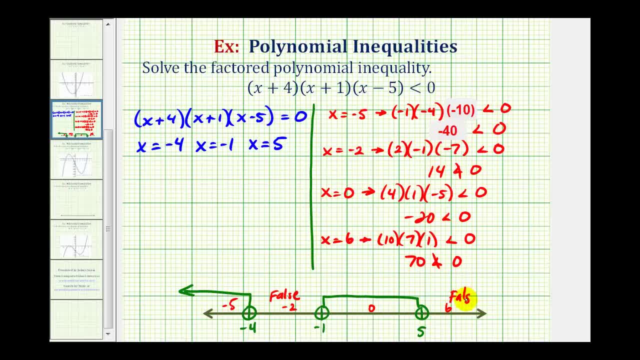 So the interval on the right here is also false Or not part of the solution. So this graph represents the x values that satisfy this inequality. Let's also give the solution using interval notation and using inequalities. So as we move to the left we approach negative infinity. 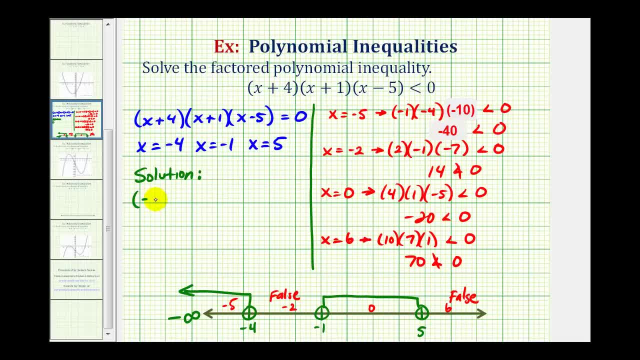 So using interval notation we'd have the interval from negative infinity to negative four. It's open on negative four because it does not include negative four. Union the open interval from negative one to positive five. Or using inequalities, we could say x is less than negative four. or 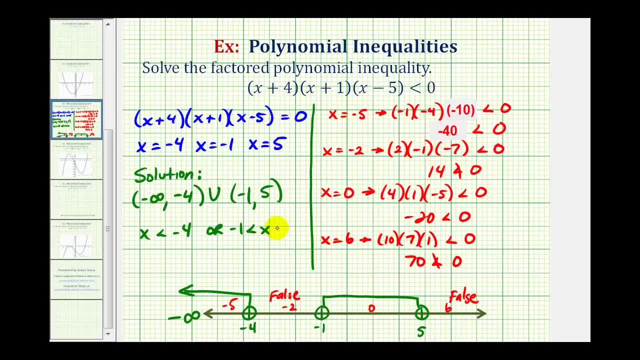 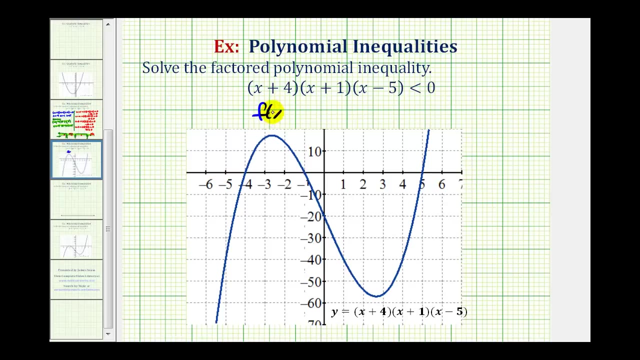 x is greater than negative, one and less than five. So we can express the solution any of these three ways: Using interval notation, using inequalities or using a graph. Let's also verify our solution graphically. To check this graphically, we want to analyze the graph of f of x. 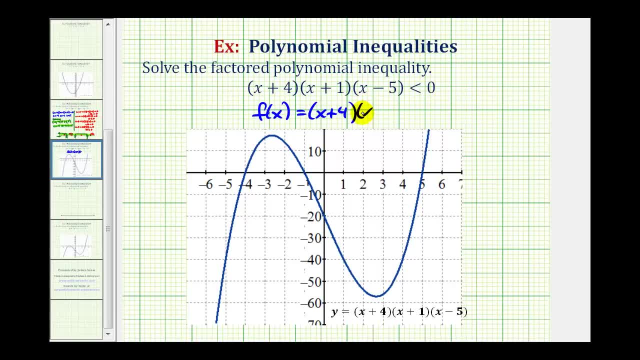 equals the quantity x plus four times the quantity x plus one times the quantity x minus five. To know when the product here is less than zero by graphing this function. we want to know when the function is less than zero. Remember, function values are y values. 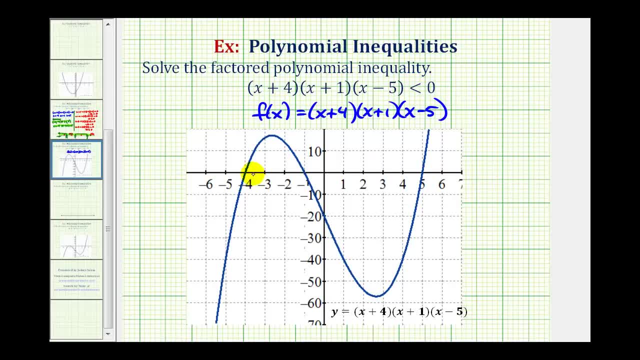 So f of x is less than zero when the y values are negative or when the function is below the x axis. Looking at the graph, notice how the function is below the x axis here and from here to here, But our solution is in terms of x.